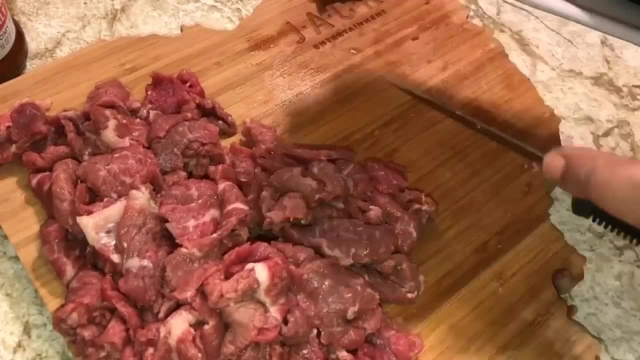 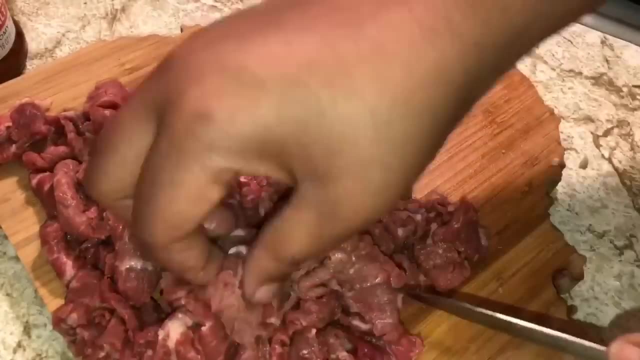 onions. It's usually seasoned with soy sauce and ginger. But then I thought to myself: hell, I don't have no ginger, so we won't be using ginger today. But it's not a- you know, a deal breaker: Still good without it. 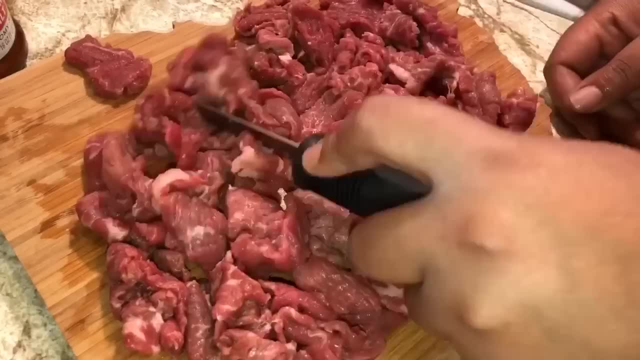 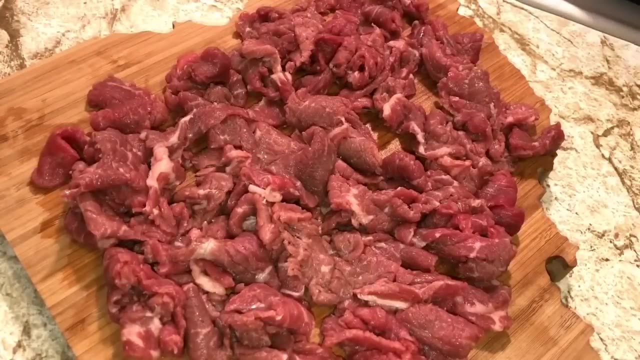 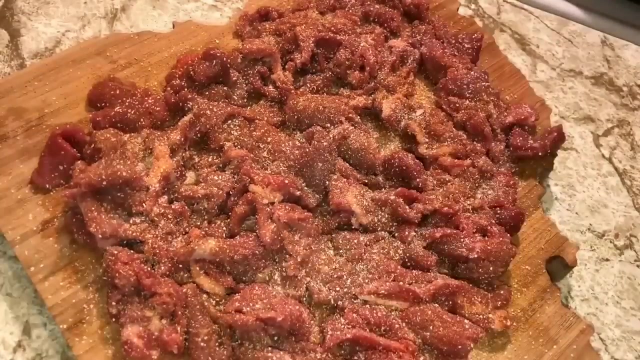 Now another- I won't say secret ingredient, but another ingredient that is, you know, traditionally added, is cornstarch. Depending on your diet, or depending on what you like or what you don't like, you know, you may use cornstarch with your pepper steak recipe. 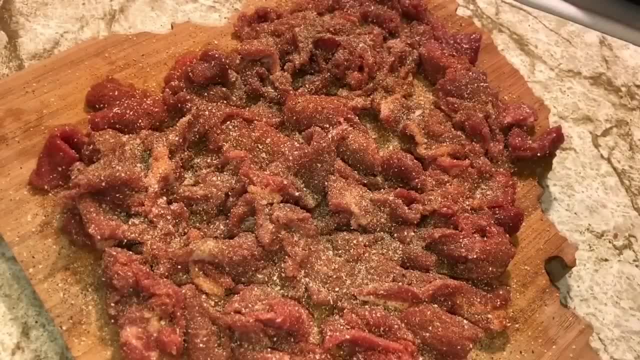 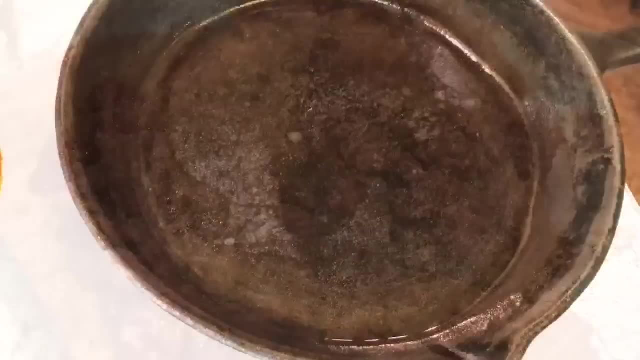 Again, a lot of people do, some people don't. But I'm seasoning the meat with salt pepper, garlic powder, onion powder, chili and a few other seasonings, as usual, And now that we got the meat seasoned, I'm buttering up. 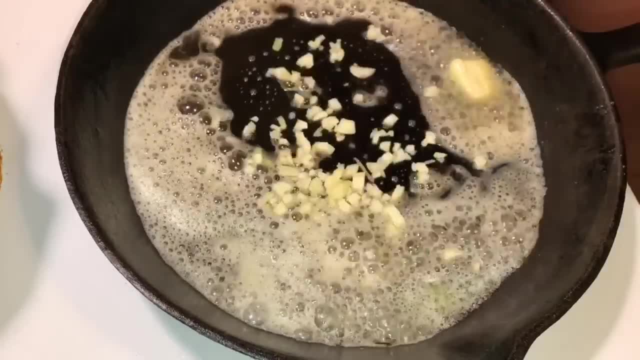 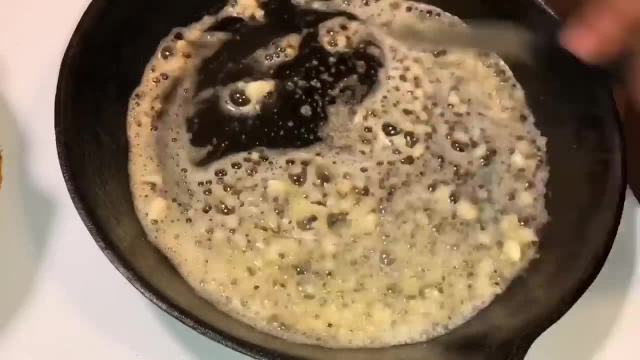 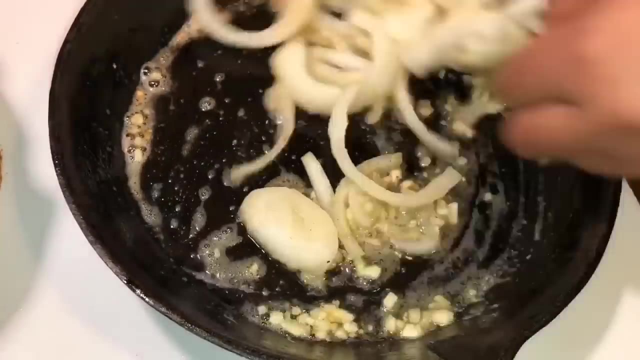 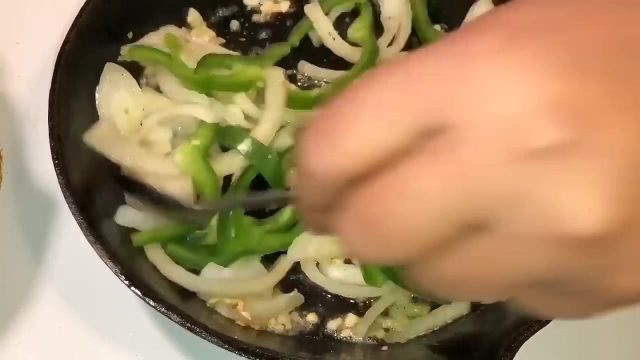 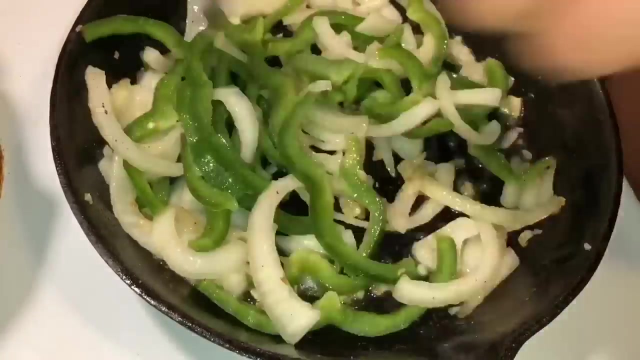 the pan so we can get the party started. Adding my garlic. but I don't want to let my garlic cook too long or get too brown, So I'm adding my onions Now. I'm adding my bell pepper. Even if you want to add a few slices of red bell pepper, you can do that also. 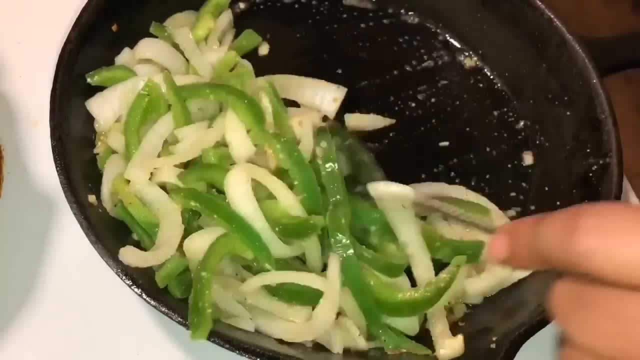 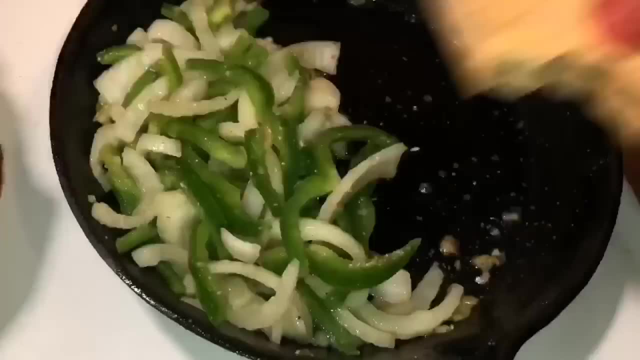 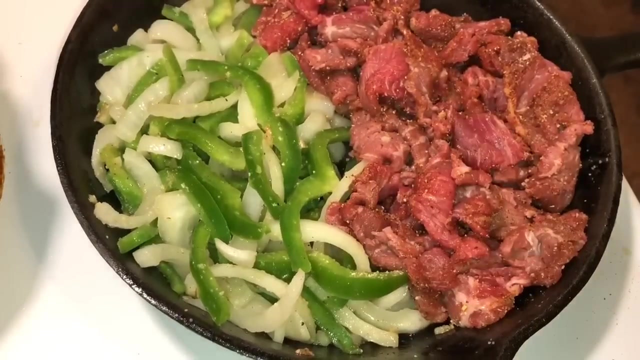 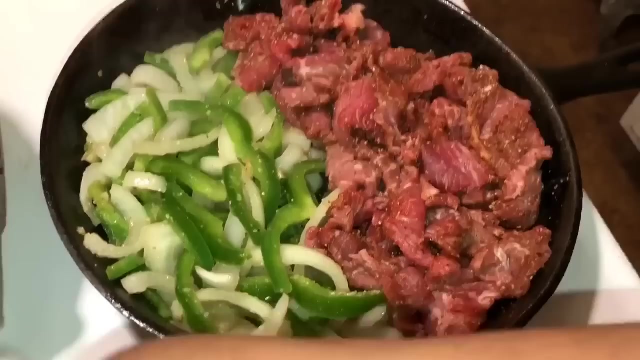 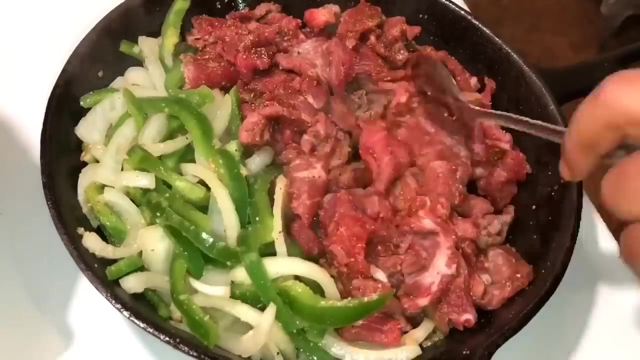 Add in a little salt. I'm definitely going to add some pepper, but I'm going to add it a little later, So don't worry about me not adding pepper right now. It's pepper steak. I know that in typical Chinese tradition they use a wok. 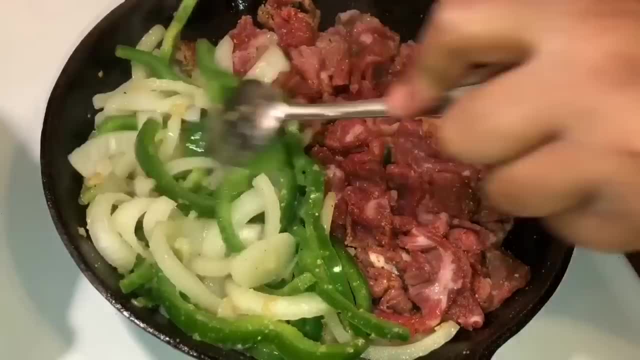 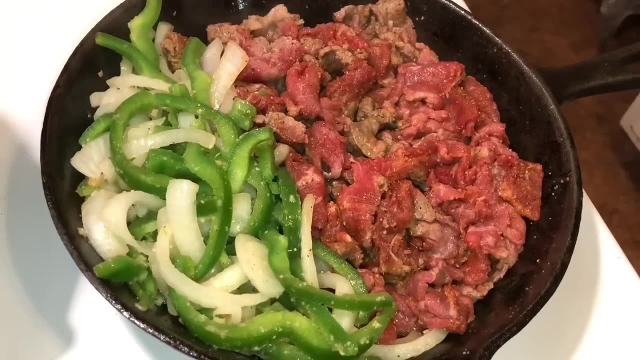 I'm not using a wok today. I'm using my favorite cast iron skillet. If I could take this skillet with me everywhere, I would Long time ago actually. ever since I can remember, my grandma has always used cast iron skillet. 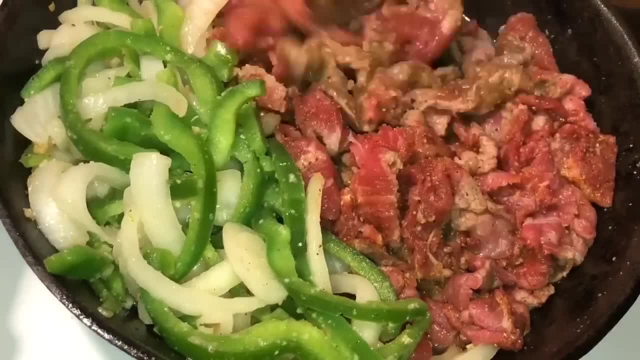 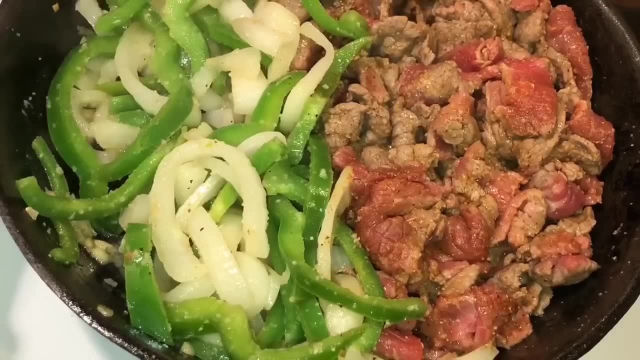 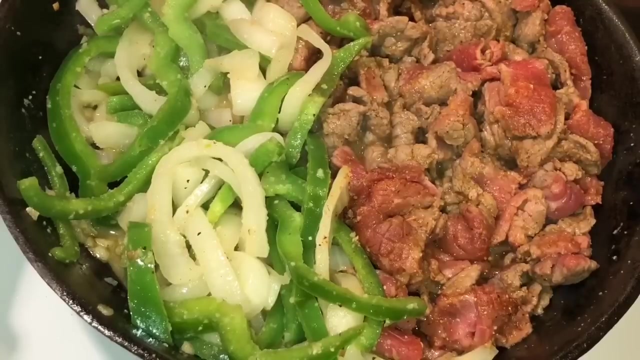 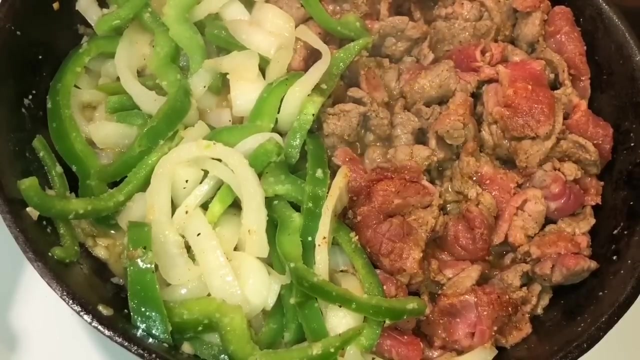 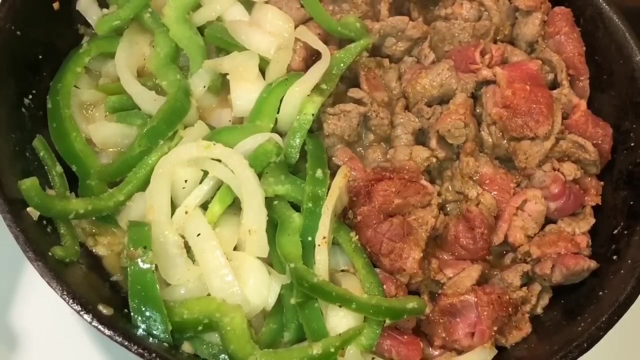 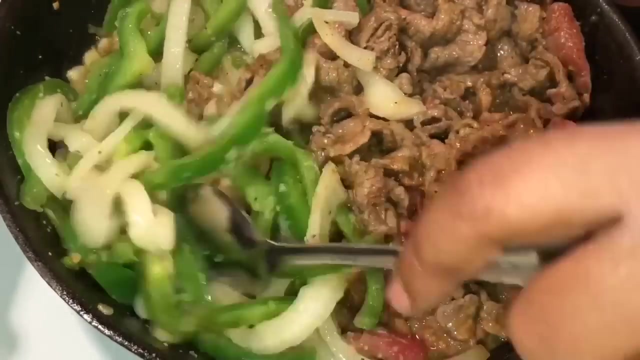 She has a set of three. Even though she's no longer here, those pots and pans are still around, So I'm just letting the meat and vegetables cook, And in a minute I'm going to stir them all up. As you can see, that's the base for our whole pepper steak. 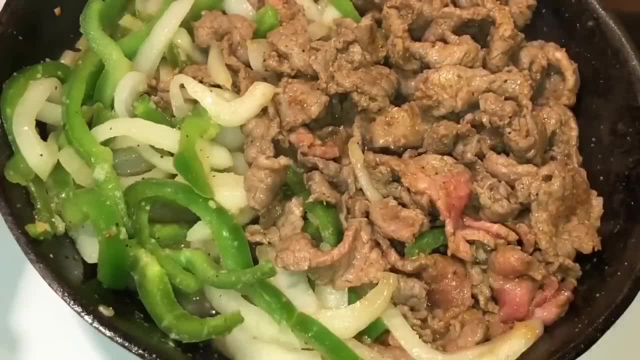 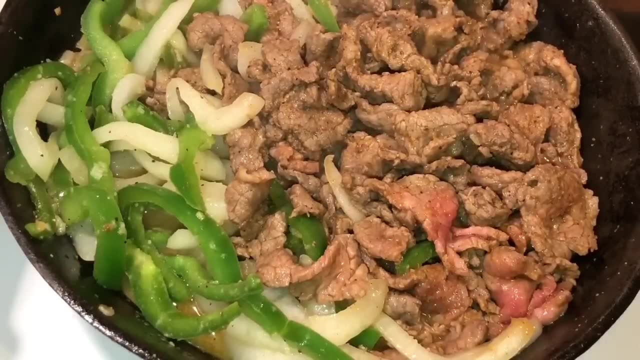 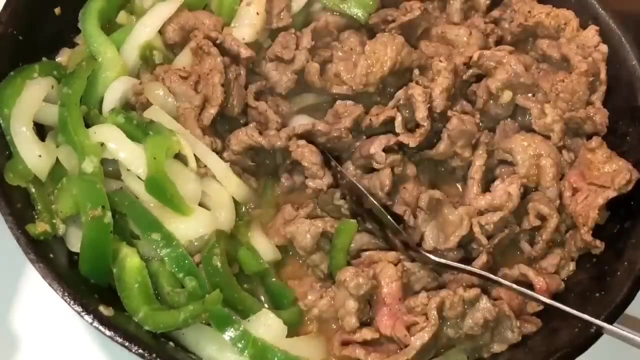 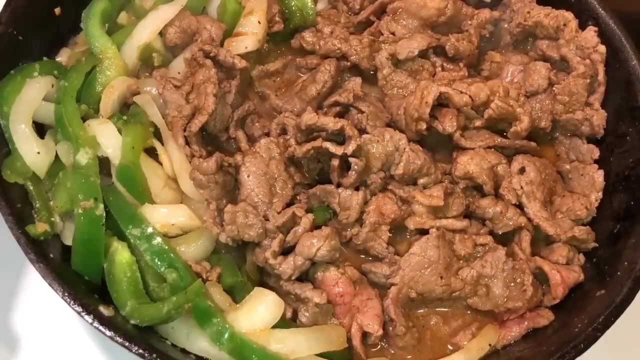 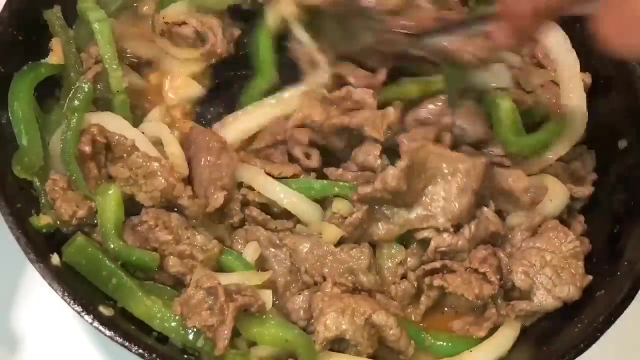 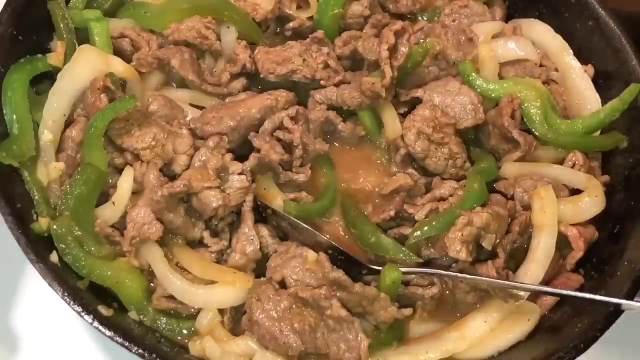 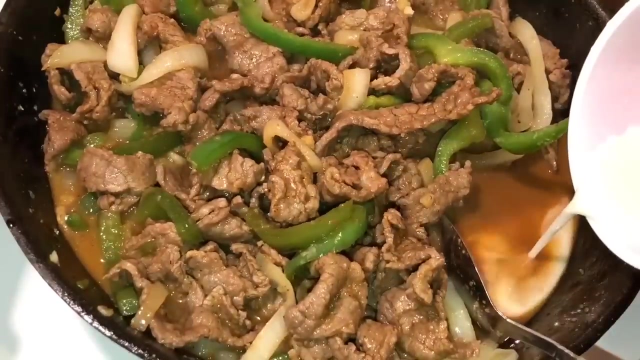 And now that my meat is brown and kind of almost done, I added in some soy sauce. And now that my meat is brown and kind of almost done, I added in some soy sauce. Add in just a little more. Now this here is the cornstarch. 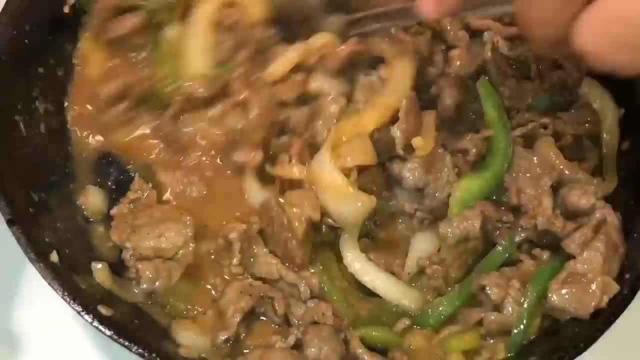 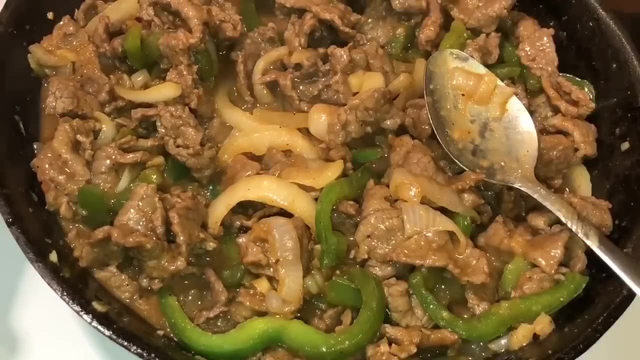 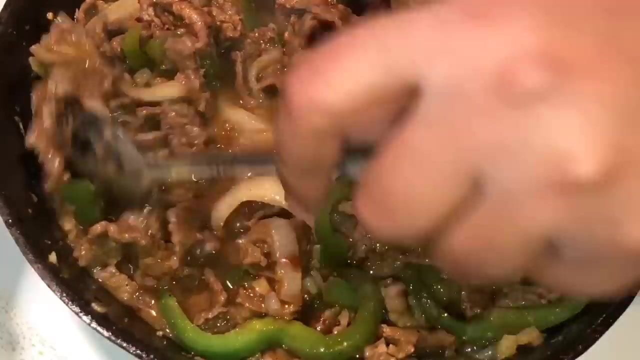 It's powdered cornstarch. You put a little in a bowl or a cup, you add cold water and you mix it up. Of course, you want to follow the instructions on the back of the package. Whatever you do, do not put warm water in the cornstarch. 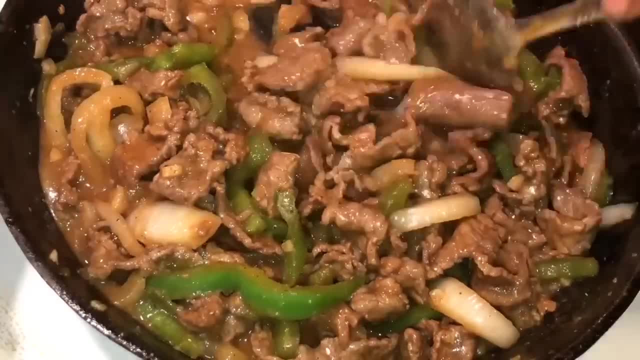 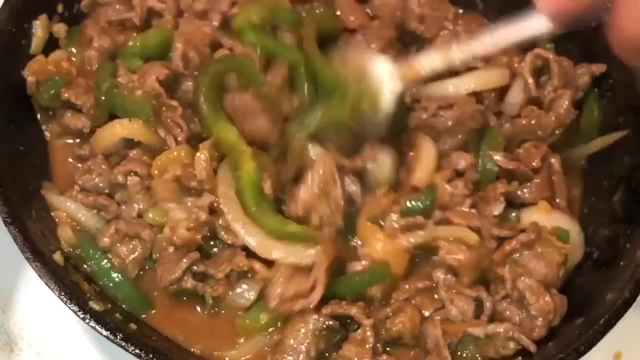 It will clump up And, as you can see, I added a little more soy sauce. I like to add as I go, whether it's seasonings, whether it's sauces, because I don't want anything to overpower the actual cornstarch. 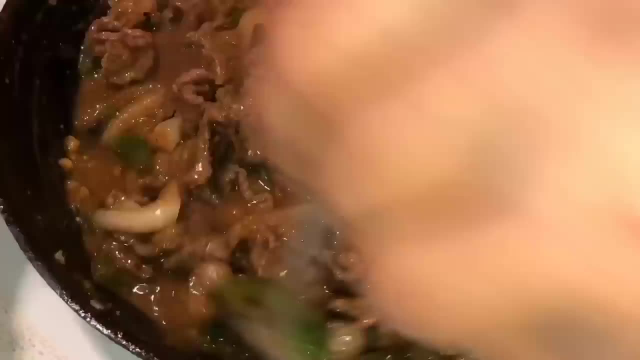 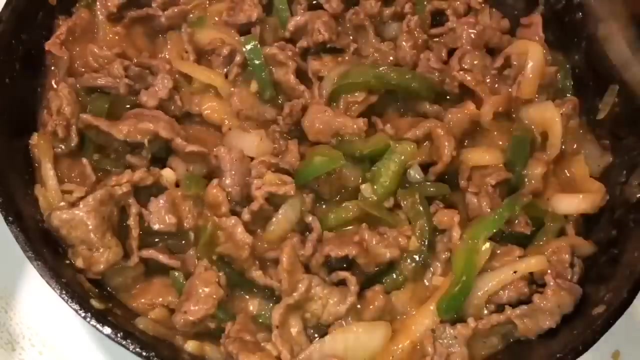 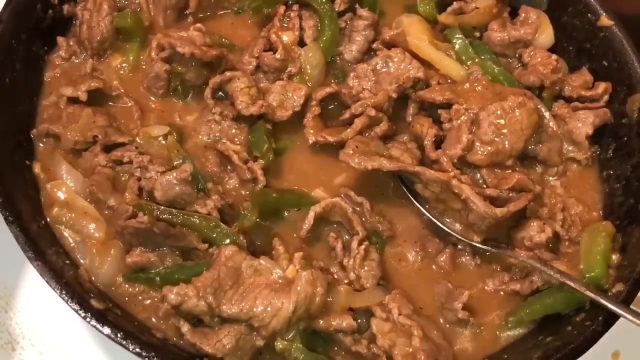 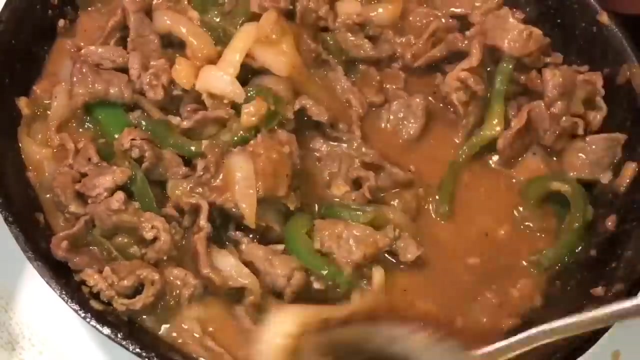 So here I'm adding just a little bit more cornstarch so I can have the sauce come together nicely. Mix it all up. That was just a little chili powder. That was just a little chili powder. I'm going to add a little more cornstarch.